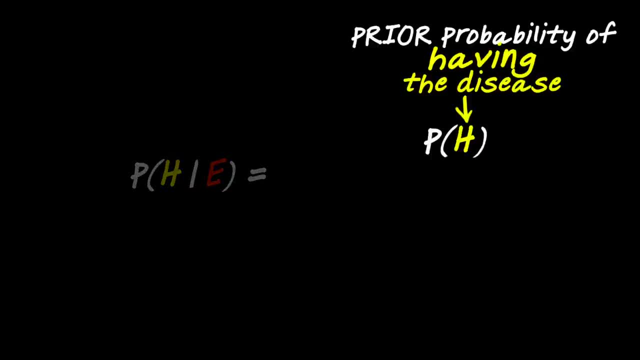 To calculate this you need to take the prior probability the hypothesis was true- that is, how likely you thought it was that you had this disease before you got the test results- and multiply it by the probability of the event, given the hypothesis is true. 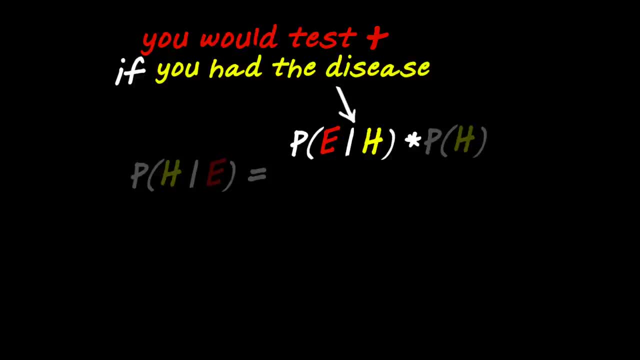 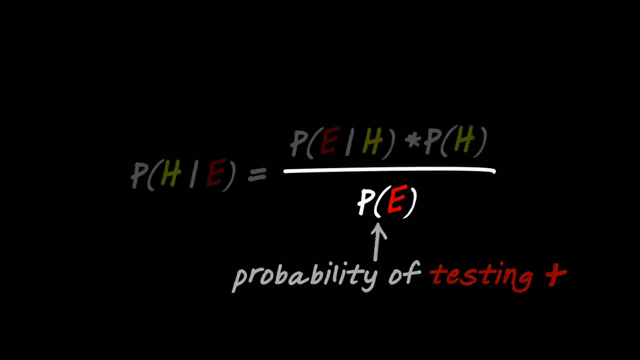 that is the probability that you would test positive if you had the disease and then divide that by the total probability of the event occurring, that is testing positive. This term is a combination of your probability of having the disease and correctly testing positive. 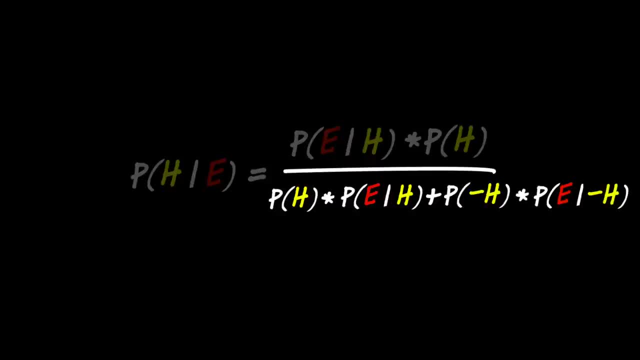 plus your probability of not having the disease and being falsely identified. The prior probability that a hypothesis is true is often the hardest part of this equation to figure out, and sometimes it's no better than a guess. But in this case a reasonable starting point is the frequency of the disease in the population. 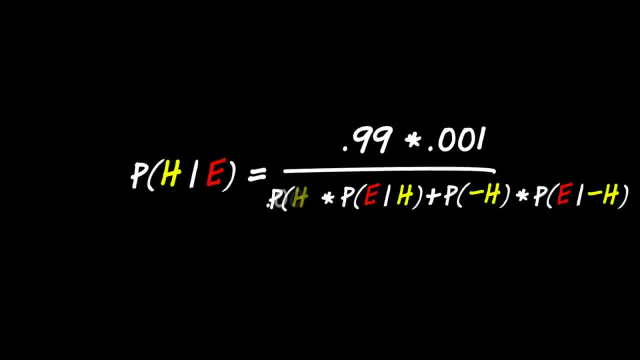 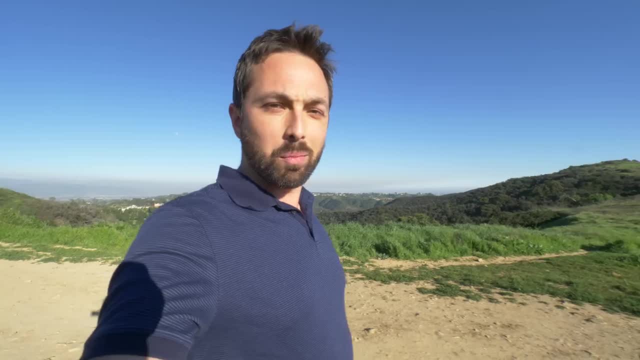 So 0.1%, And if you plug in the rest of the numbers, you find that you have a 9% chance of actually having the disease after testing positive, Which is incredibly low if you think about it. Now, this isn't some sort of crazy magic. 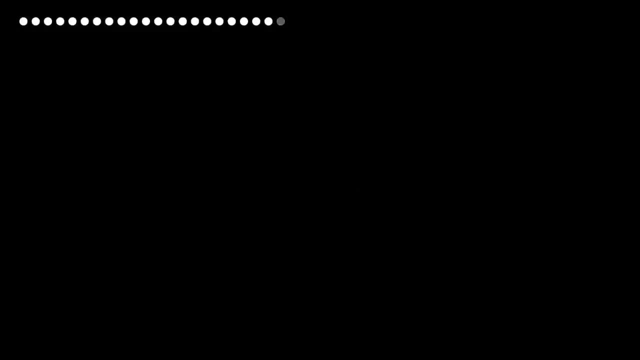 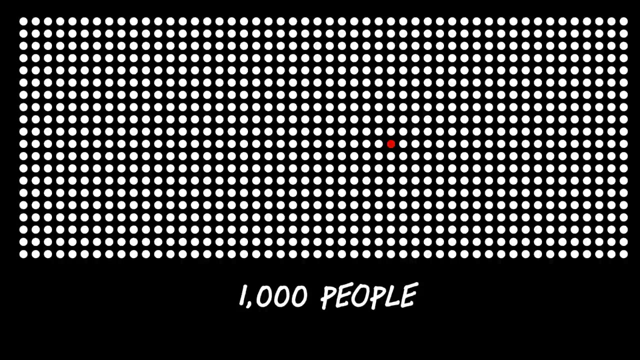 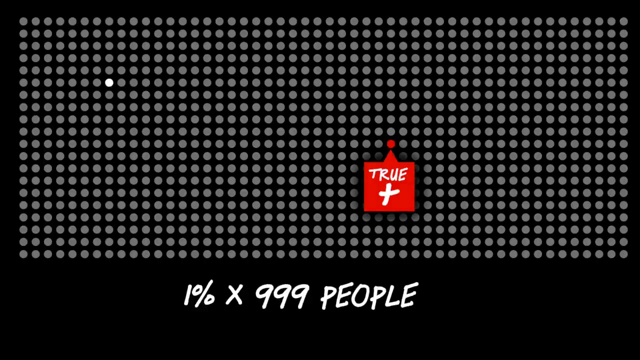 It's actually common sense applied to mathematics. Just think about a sample size of a thousand people. Now, one person out of that thousand is likely to actually have the disease and the test would likely identify them correctly as having the disease. But out of the 999 other people, 1% or 10 people would falsely be identified as having the disease. 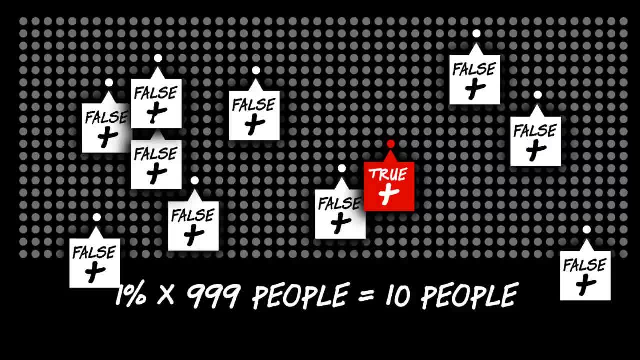 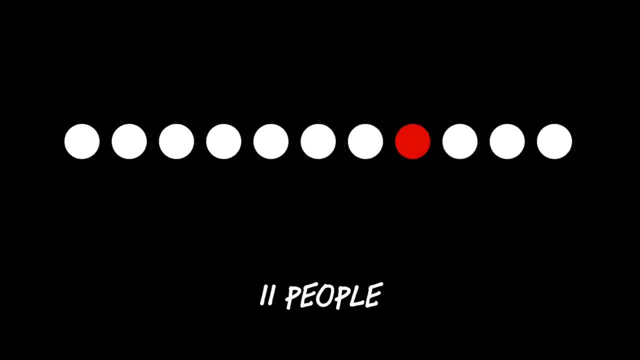 So if you're one of those people who has a positive test result and everyone's just selected at random, well, you're actually part of a group of 11 where only one person has the disease, So your chances of actually having it are 1 in 11.. 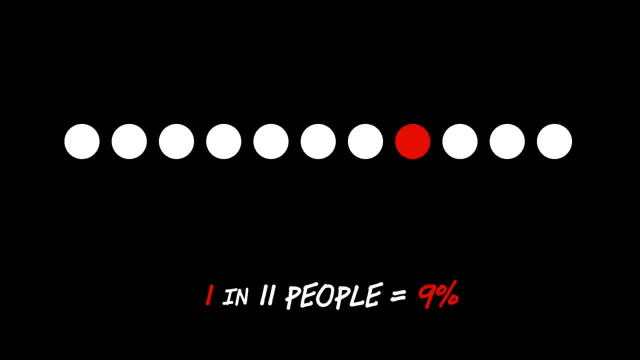 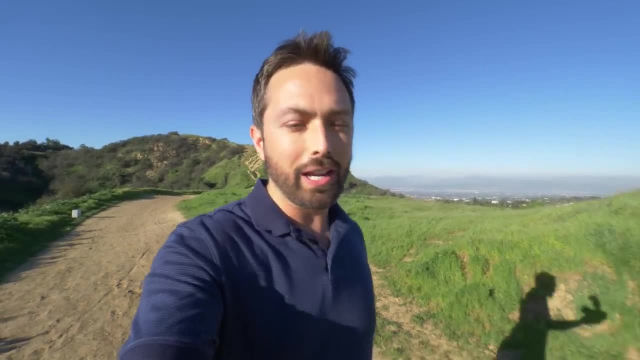 9%. It just makes sense. When Bayes first came up with this theorem, he didn't actually think it was revolutionary. He didn't even think it was worthy of publication. He didn't submit it to the Royal Society of which he was a member. 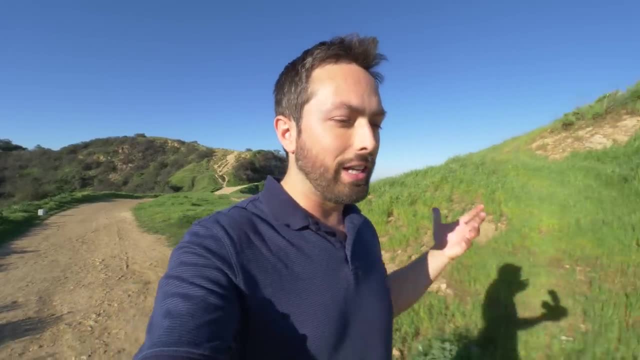 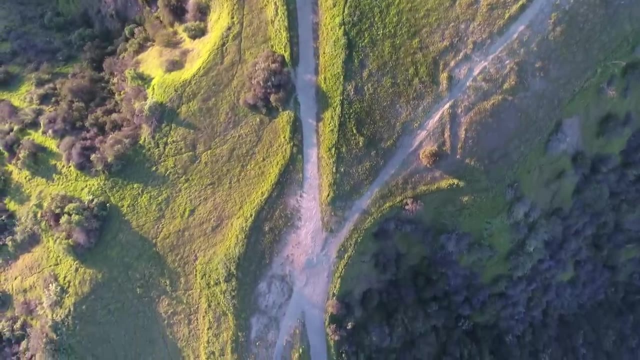 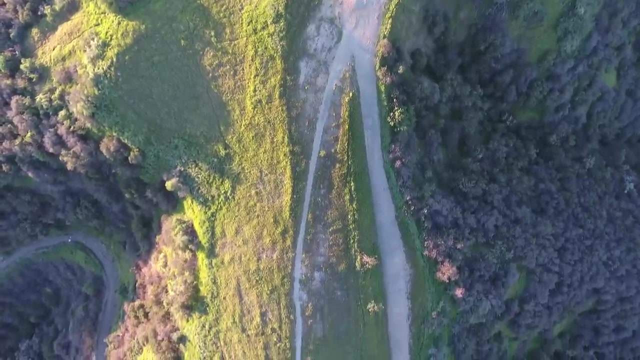 And in fact it was discovered in his papers. after he died- and he had abandoned it for more than a decade, His relatives asked his friend Richard Price to dig through his papers and see if there was anything worth publishing in there, And that's where Price discovered what we now know as the origins of Bayes' theorem. 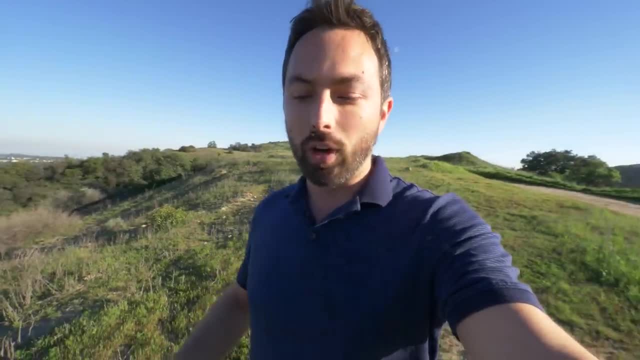 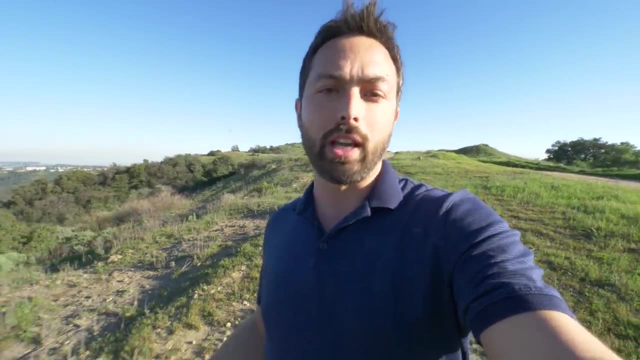 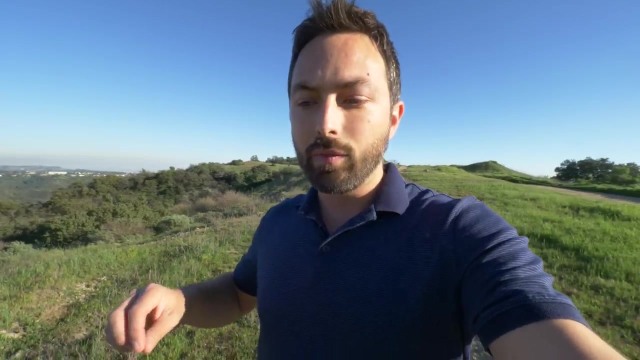 Bayes originally considered a disease. It was a thought experiment where he was sitting with his back to a perfectly flat, perfectly square table and then he would ask an assistant to throw a ball onto the table. Now, this ball could obviously land and end up anywhere on the table, and he wanted to figure out where it was. 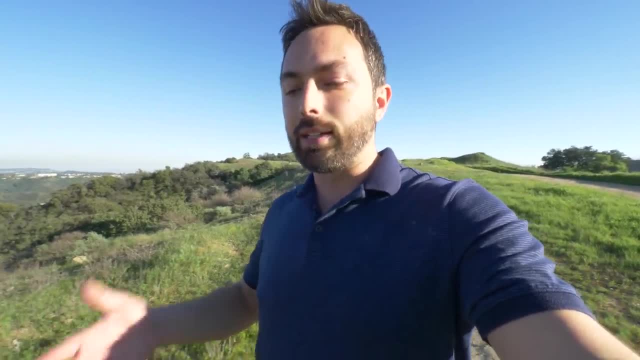 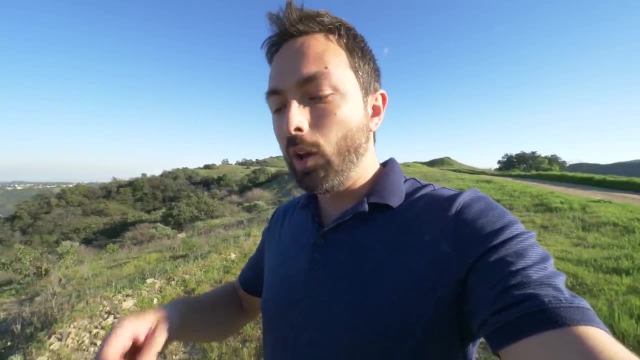 So what he'd ask his assistant to do was throw on another ball and then tell him if it landed to the left or to the right or in front behind of the first ball, And he would note that down and then ask for more and more balls to be thrown on the table. 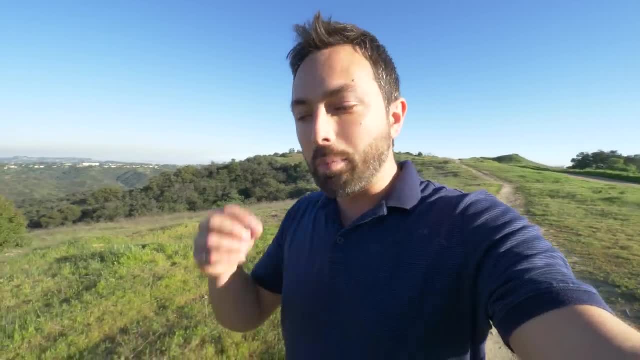 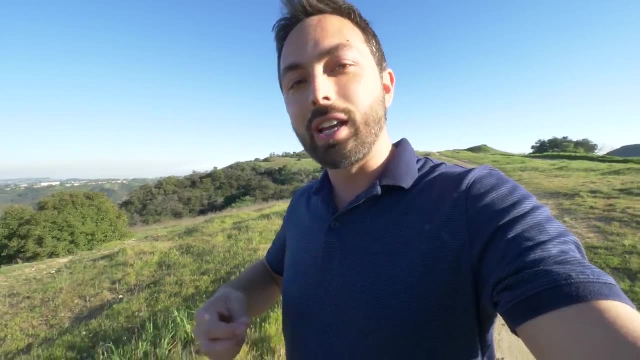 What he realized was that through this method, he could keep updating his idea of where the first ball was Now. of course, he would never be completely certain, but with each new piece of evidence he would get more and more accurate. 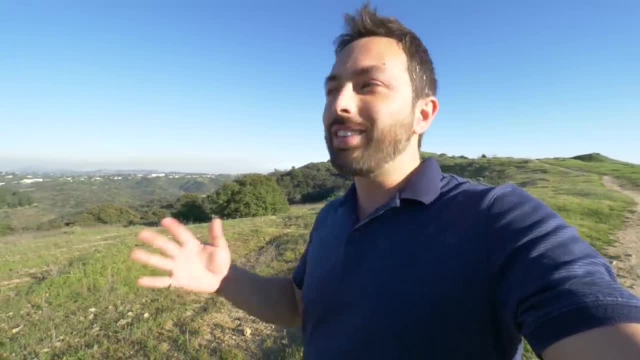 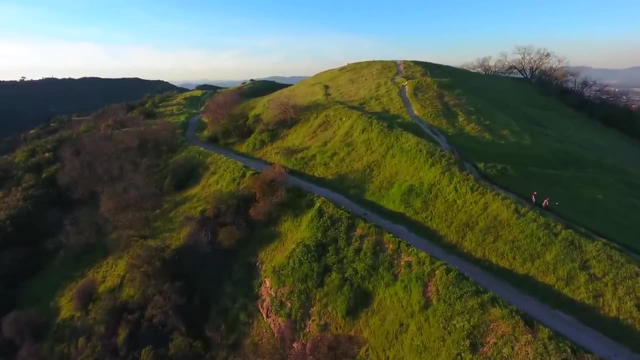 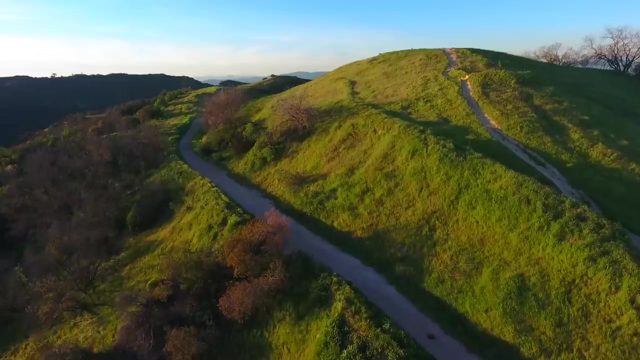 And that's how Bayes saw the world. It wasn't that he thought the world was not determined, that reality didn't quite exist, but it was that we couldn't know it perfectly, And all we could hope to do was update our understanding as more and more evidence became available. 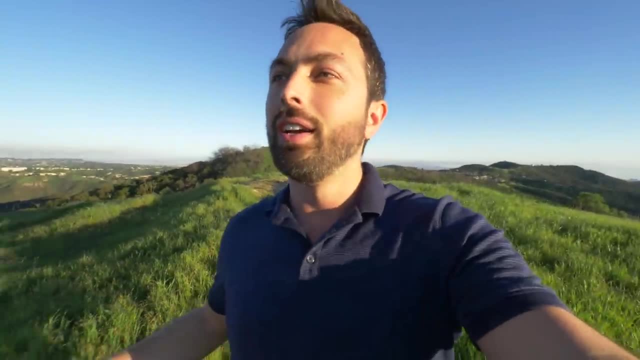 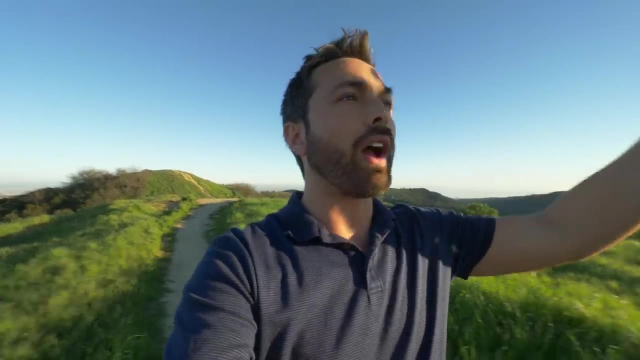 When Richard Price introduced Bayes' theorem, he made an analogy to a man coming out of a cave. Maybe he'd lived his whole life in there and he saw the sun rise for the first time and kind of thought to himself: is this a one-off, Is this a quirk? 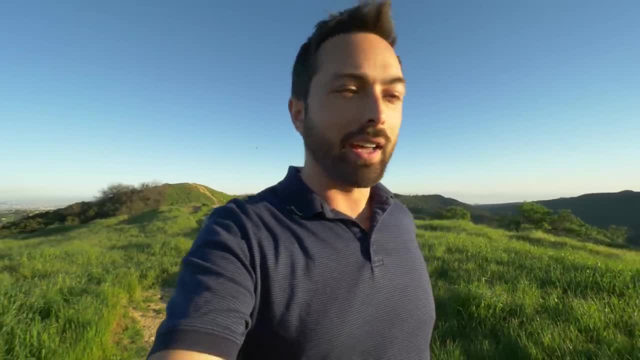 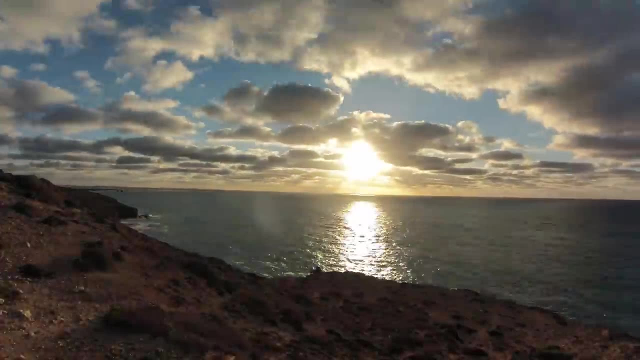 Or does the sun always do this And then every day after that, as the sun rose again, he could get a little bit more confident that, well, that was the way the world works. So Bayes' theorem wasn't really a formula intended to be used just once. 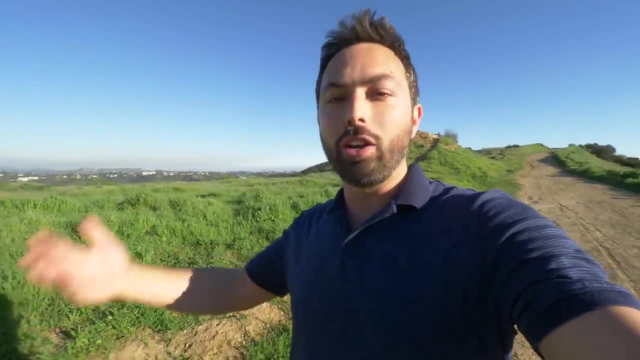 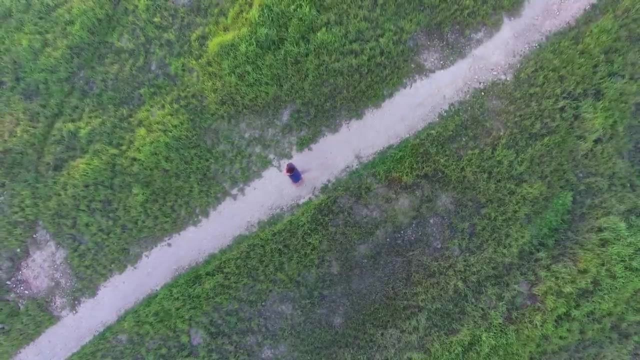 It was intended to be used multiple times, each time gaining new evidence and updating your probability that something is true. So if we go back to the first example, when you tested positive for a disease, what would happen if you went to another doctor, get a second opinion and get that test run again? 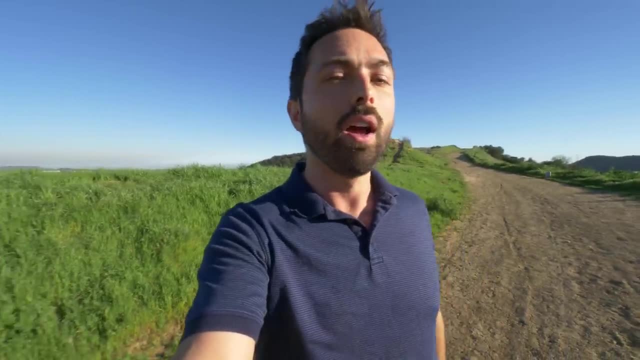 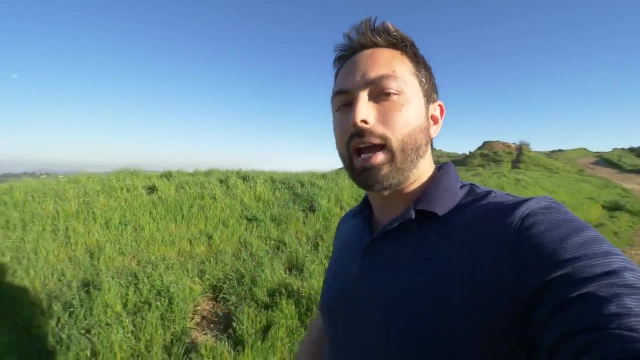 but let's say by a different lab, just to be sure that those tests are independent. And let's say that test also comes back as positive. Now what is the probability that you actually have the disease? Well, you can use Bayes' formula again. 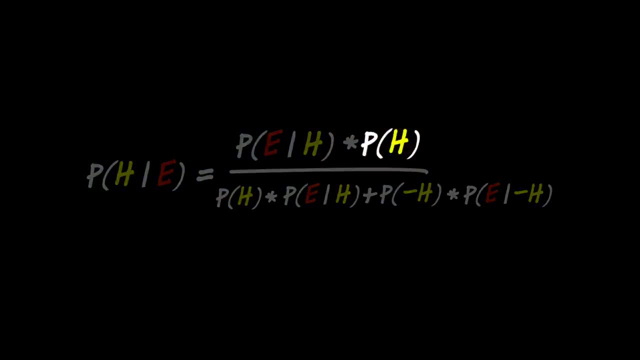 except this time for your prior probability that you have the disease. you have to put in the posterior probability, the probability that we worked out before, which is 9%, because you've already had one positive test. And if you crunch those numbers, 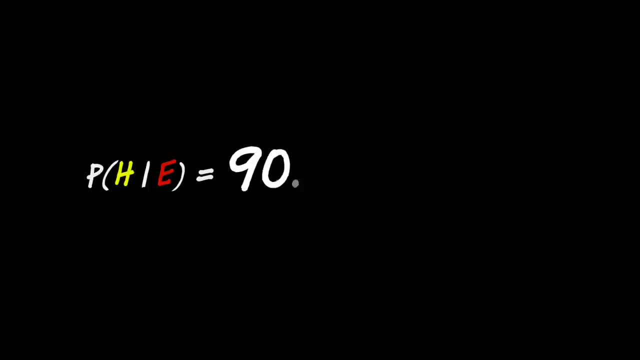 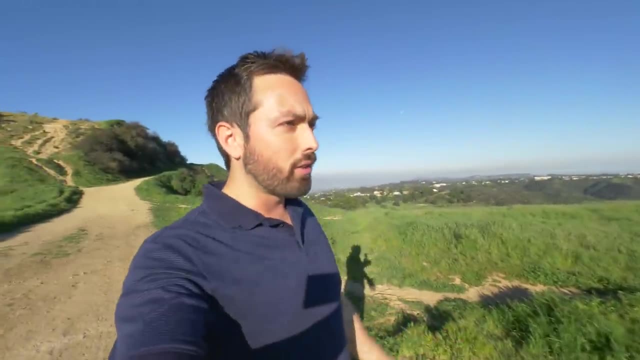 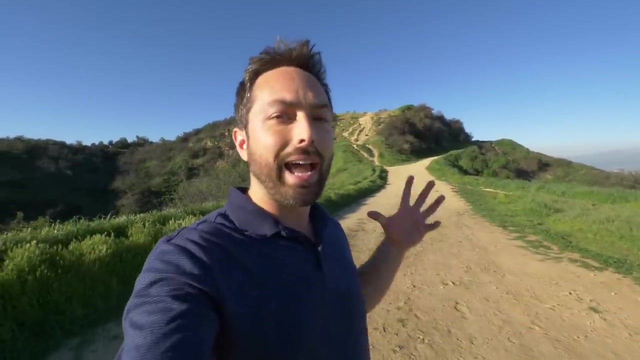 the new probability based on two positive tests is 91%. There's a 91% chance that you actually have the disease, which kind of makes sense. Two positive results by different labs are unlikely to just be chance, But you'll notice that probability is still not as high as the accuracy. 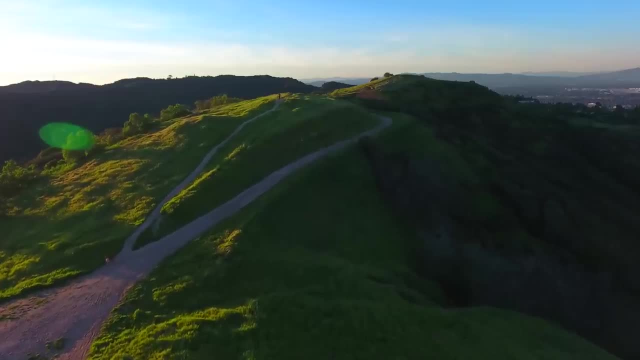 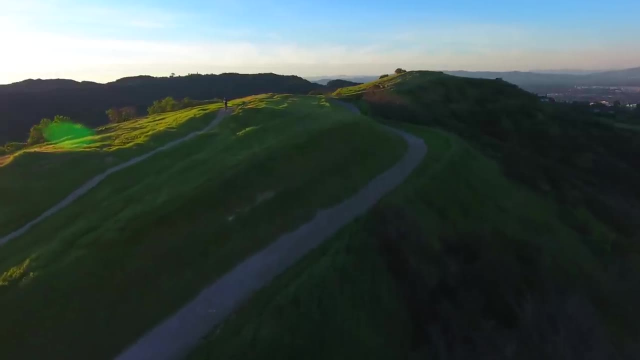 the reported accuracy of the test Bayes' theorem has found a number of practical applications, including, notably, filtering your spam. You know traditional spam filters actually do a kind of bad job. There's too many false positives. too much of your email ends up in spam. 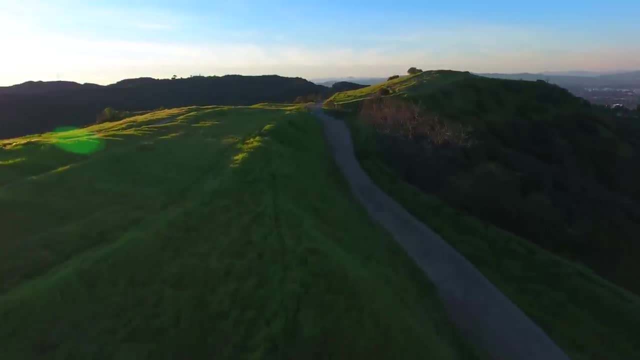 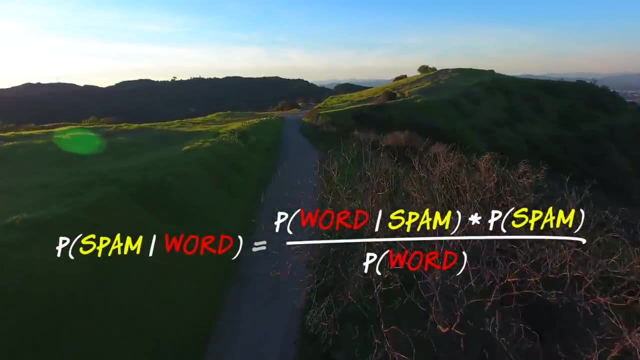 But using a Bayesian filter, you can look at the various words that appear in emails and use Bayes' theorem to give a probability that the email is spam, given that those words appear Now. Bayes' theorem tells us how to update our beliefs in light of new evidence. 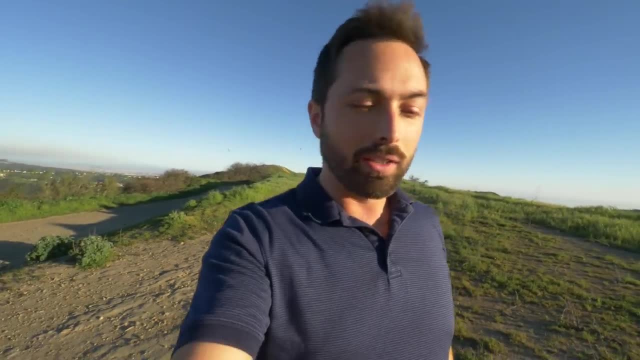 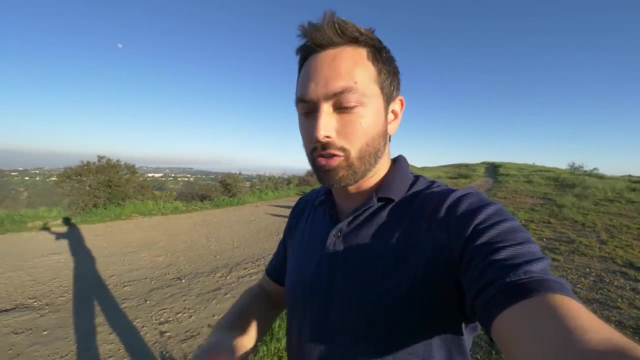 But it can't tell us how to set our prior beliefs, And so it's possible for some people to hold that certain things are true with 100% certainty and other people to hold those same things are true with 0% certainty. What Bayes' theorem shows us is that 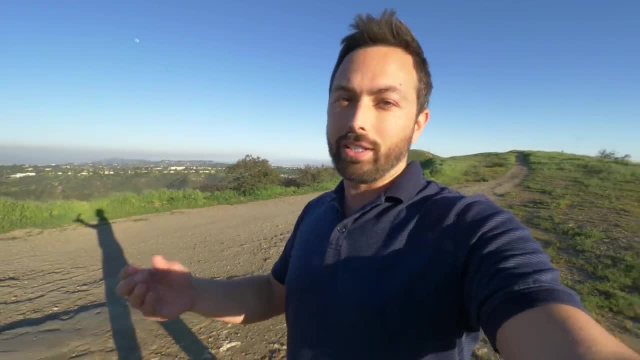 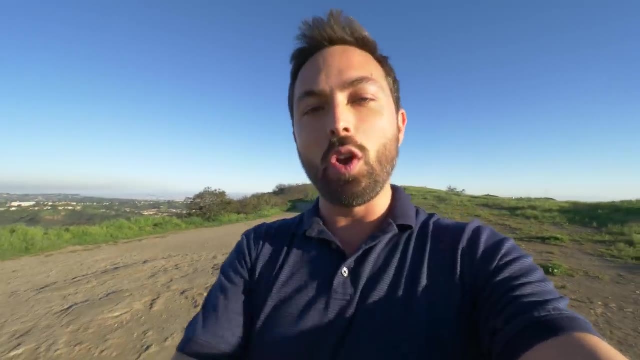 in those cases, there is absolutely no evidence, nothing anyone could do to change their minds, And so, as Nate Silver points out in his book The Signal and the Noise, we should probably not have debates between people with 100% prior certainty and 0% prior certainty. 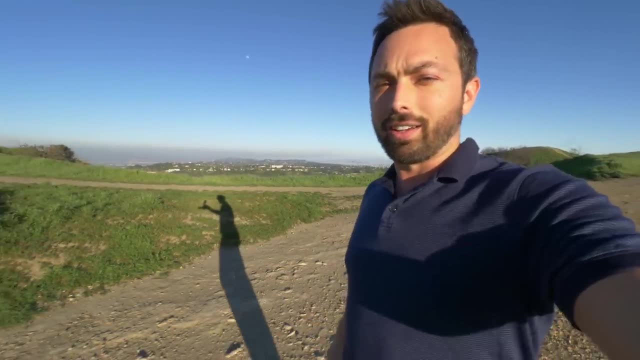 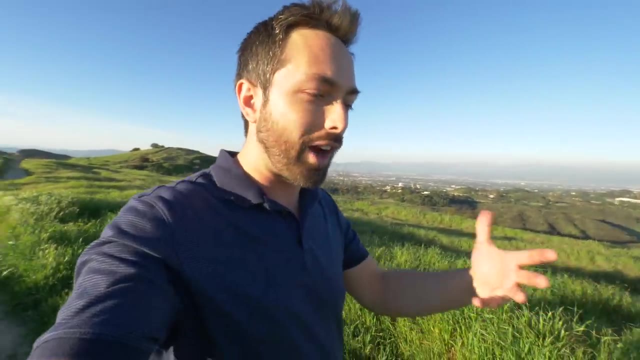 because, well, really, they'll never convince each other of anything. Most of the time when people talk about Bayes' theorem, they discuss how counterintuitive it is and how we don't really have an inbuilt sense of it. 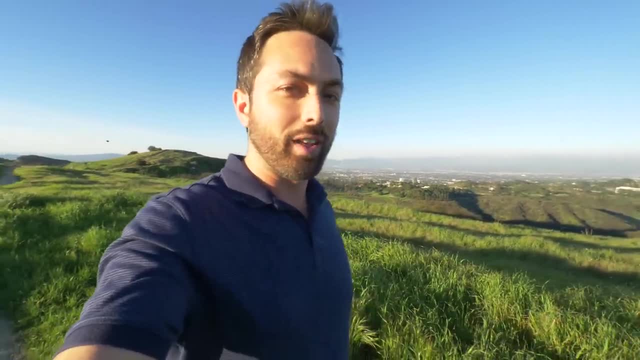 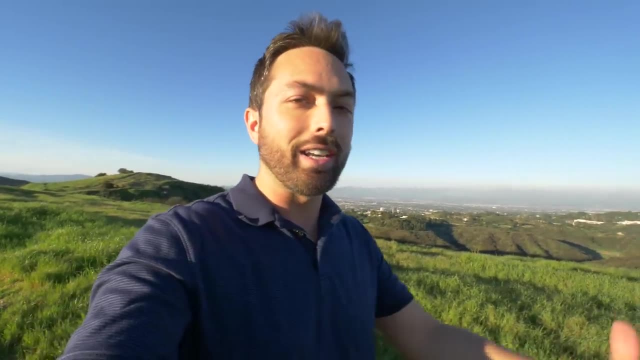 But recently my concern has been the opposite, that maybe we're too good at internalizing the thinking behind Bayes' theorem. And the reason I'm worried about that is because I think in life we can get used to particular circumstances. we can get used to results. 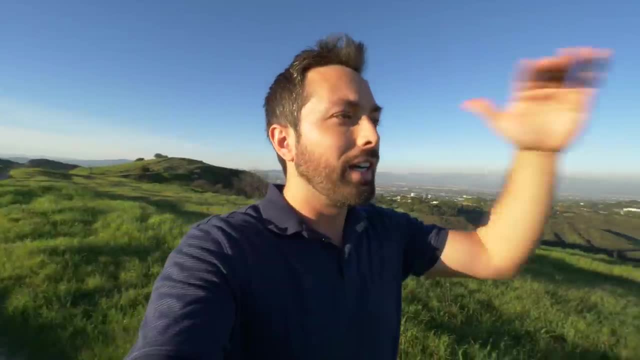 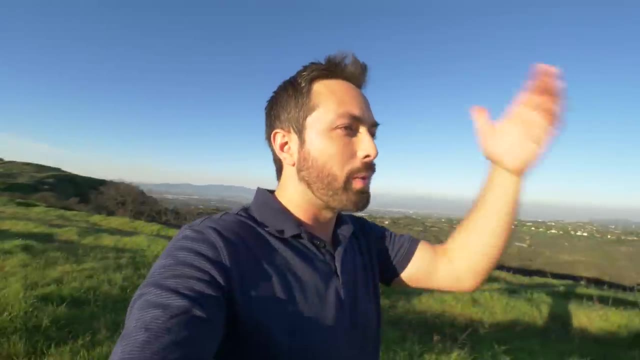 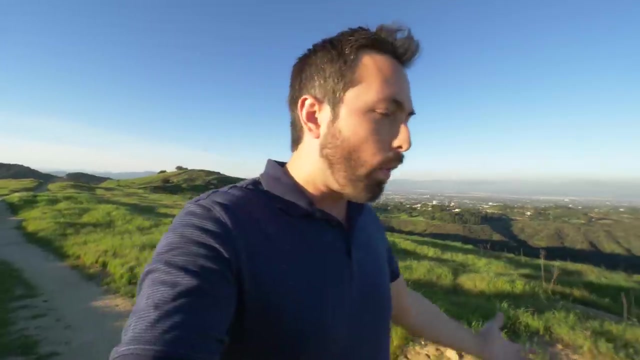 maybe getting rejected or failing at something or getting paid a low wage, and we can internalize that as though we are that man emerging from the cave and we see the sun rise every day and every day, and we keep updating our beliefs to a point of near certainty. 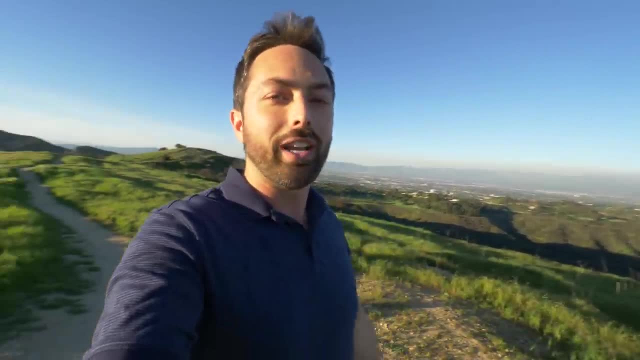 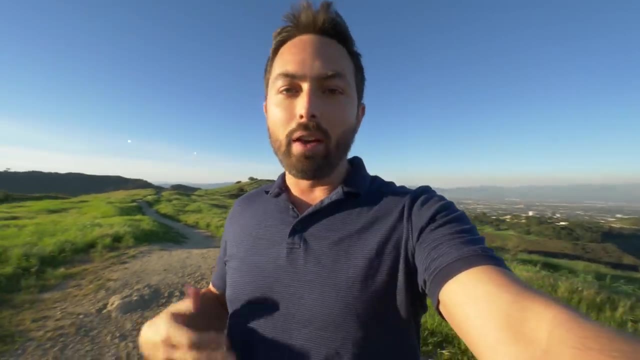 that we think that that is basically the way that nature is. It's the way the world is and there's nothing that we can do to change it. You know, there's Nelson Mandela's quote that everything is impossible until it's done. 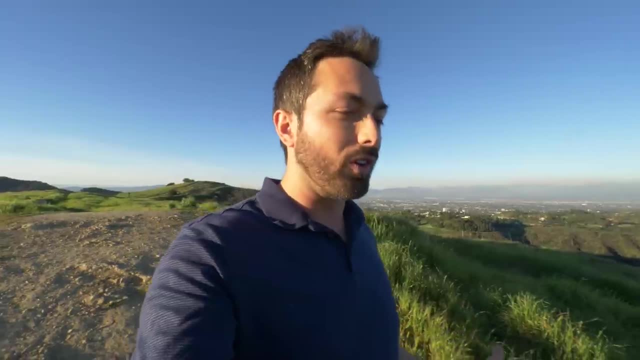 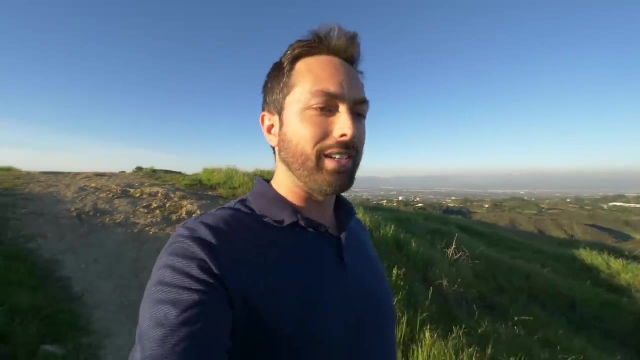 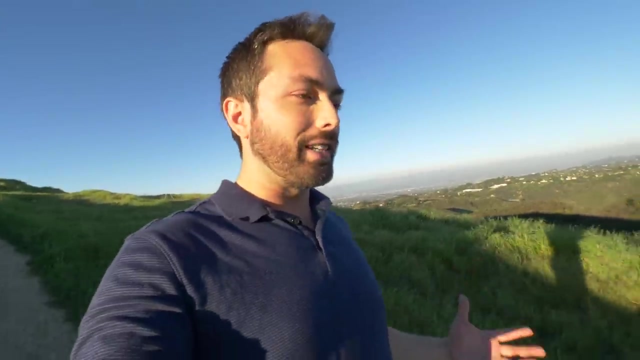 And I think that is kind of a very Bayesian viewpoint on the world. If you have no instances of something happening, then what is your prior for that event? It will seem completely impossible. Your prior may be zero until it actually happens. You know the thing we forget in Bayes' theorem. 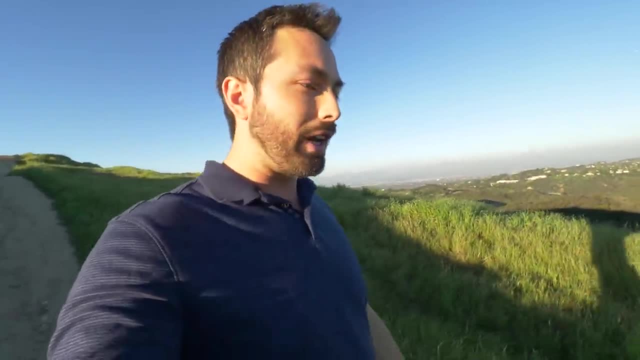 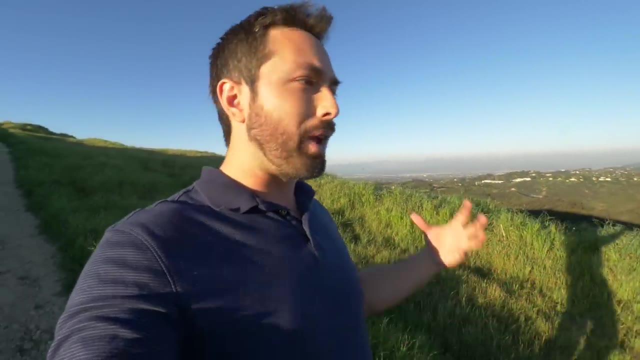 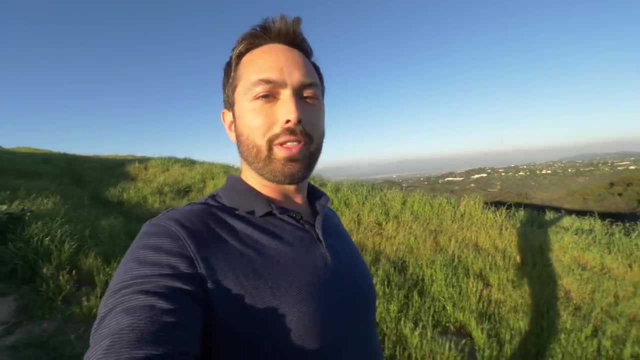 is that our actions play a role in determining outcomes and determining how true things actually are. But if we internalize that something is true- and maybe we're 100% sure that it's true and there's nothing we can do to change it- well then we're going to keep on doing the same thing. 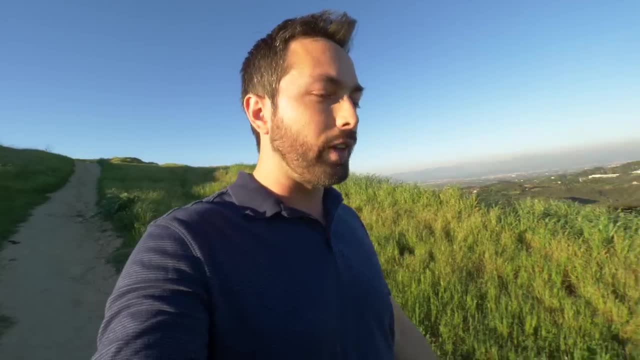 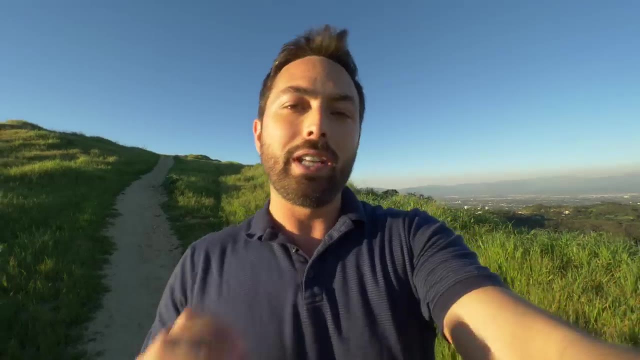 and we're going to keep on getting the same result. It's a self-fulfilling prophecy. So I think a really good understanding of Bayes' theorem implies that experimentation is essential If you've been doing the same thing for a long time. 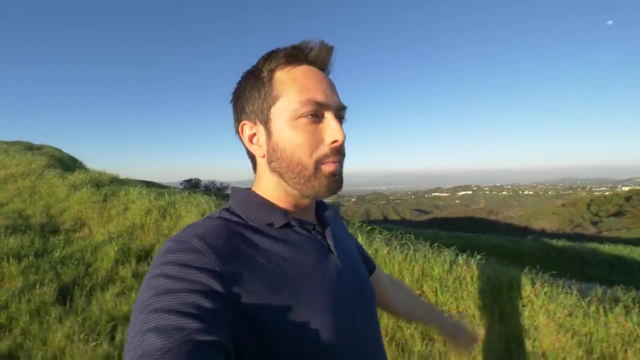 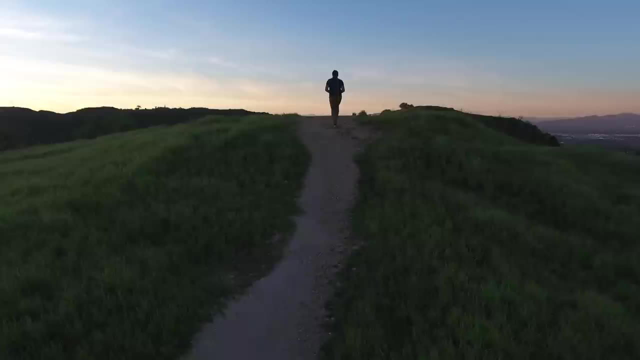 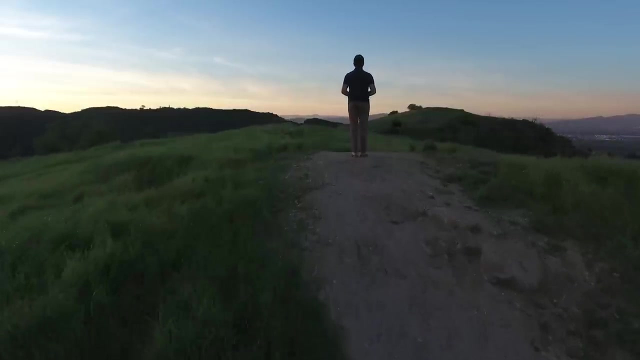 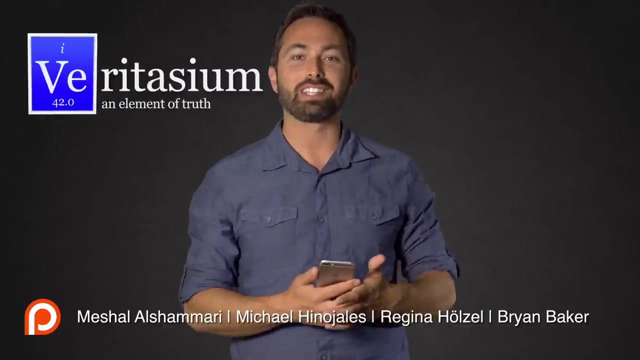 and getting the same result that you're not necessarily happy with. maybe it's time to change. So is there something like that that you've been thinking about? If so, let me know in the comments. Hey, this episode of Veritasium was supported in part by viewers like you on Patreon and by Audible. 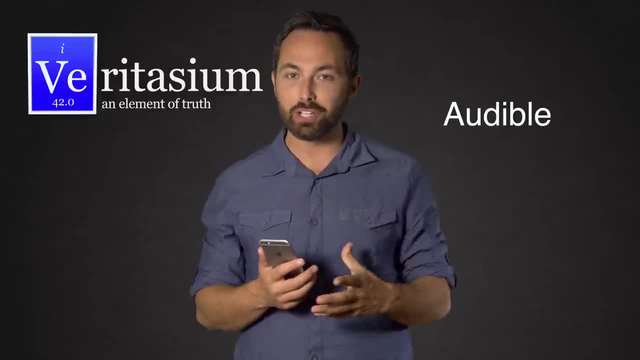 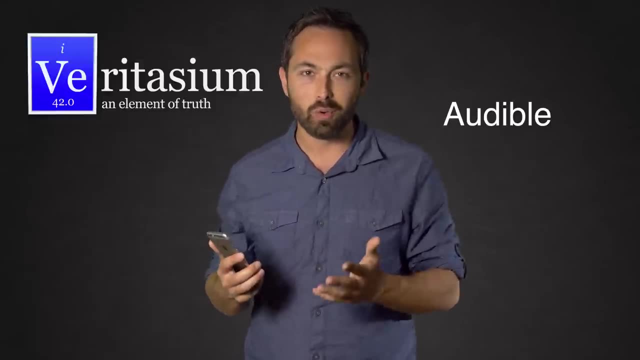 Audible is a leading provider of spoken audio information, including an unmatched selection of audiobooks, original programming, news, comedy and more. So if you're thinking about trying something new and you haven't tried Audible yet, you should give them a shot. 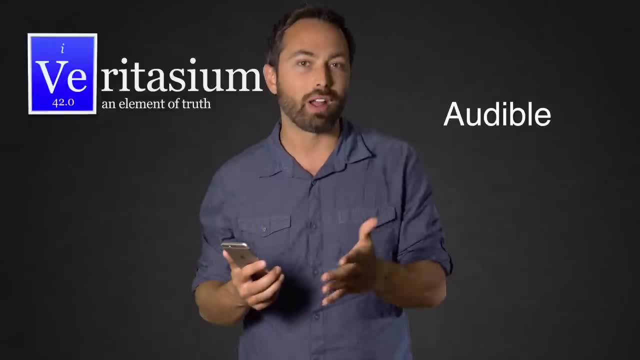 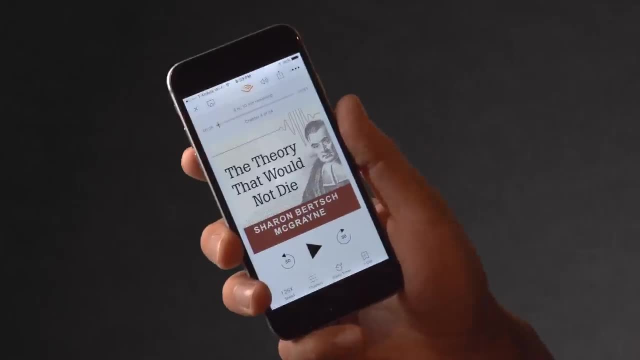 And for viewers of this channel they offer a free 30-day trial just by going to audiblecom. slash veritasium. You know, the book I've been listening to on Audible recently is called The Theory That Would Not Die, by Cheryl Birch McGrain.